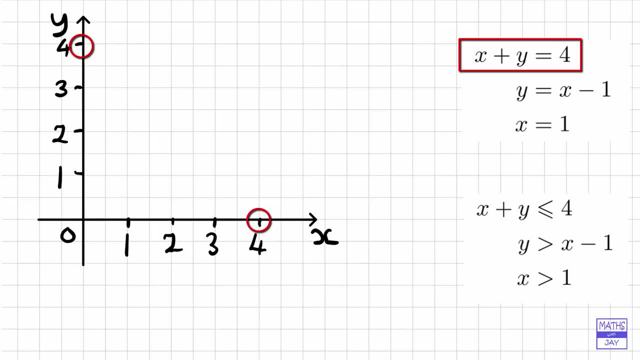 around. when y is four, x is zero. but another way of doing it is just to plot a few points. so, for example, you could choose: when x is one, what would y be? well, y would be three. when x is two, what would y be? y would be two, and so on. so let's just draw that line. 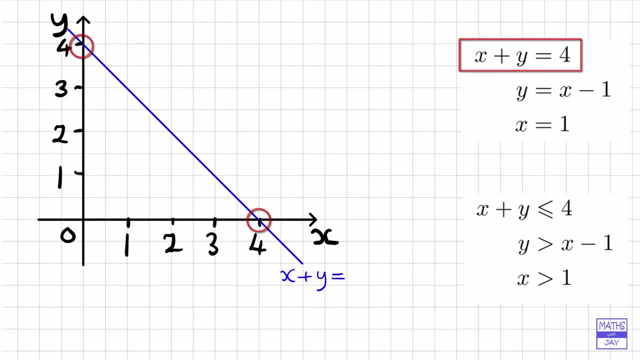 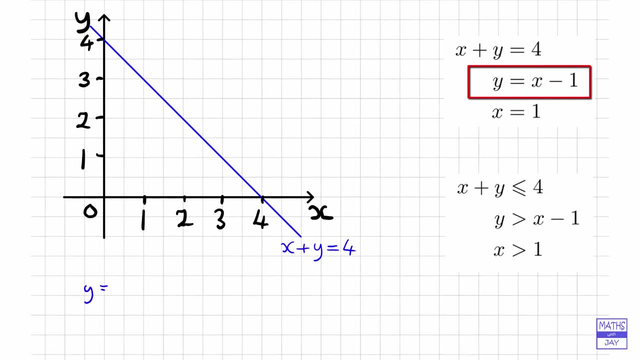 so there we've got. x plus y equals four. then let's think about the next line. so there we've got y equals x minus one. so one way of doing this one would be to choose a value for x and then work out what y is. so, for example, if x is two, then y is two minus one, so that's one. 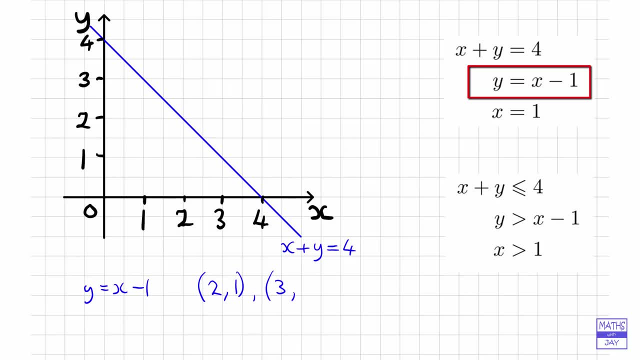 and if x is three, y will be three minus one, so that will be two and you only actually need two points for a straight line, but it's a good idea to do three just as a check. so if x is four, then y will be three. so those points are going to be two. one 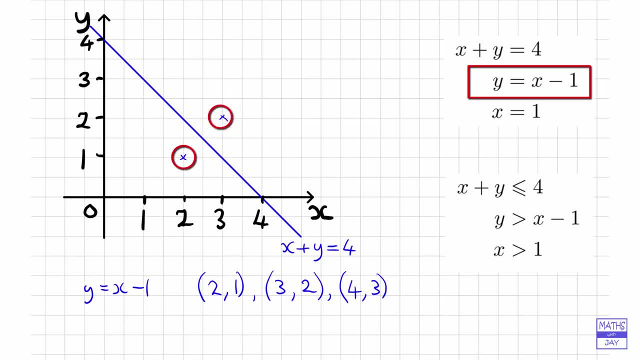 three, two and four, three, and then we just join those points and extend it in both directions. another way of thinking about drawing that line would be to say: well, we know that line is of the form: y equals mx plus c, and m is the gradient and m is the number multiplying the x. so that's one. 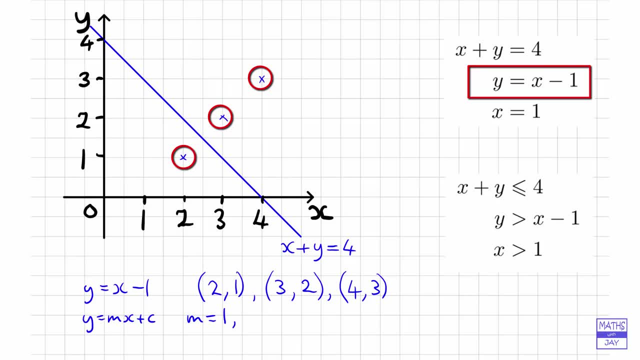 so we know that for every one along we're going up one, and we know that c is equal to minus one and that's where the graph cuts the, the y-axis, just about c. negative one on our graph, can't we? we can write it in there, so that's another way of drawing this. 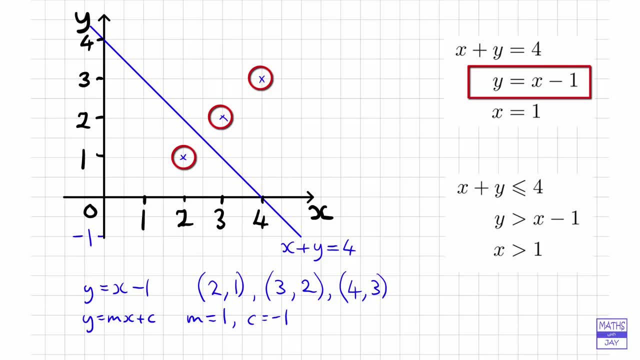 graph. whichever way you choose, it should come out to be the same thing. so that's the line: y equals x minus one. and then the last line is the simplest one, i think, because it's just x equals one. so we want the line where x minus one is quantity 1 over 1. that's the formula we're going to make for total of x minus 1.. 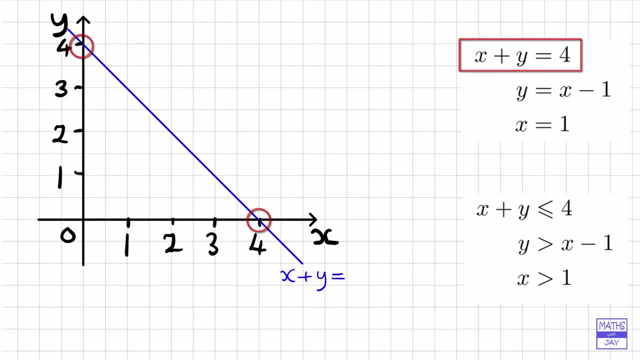 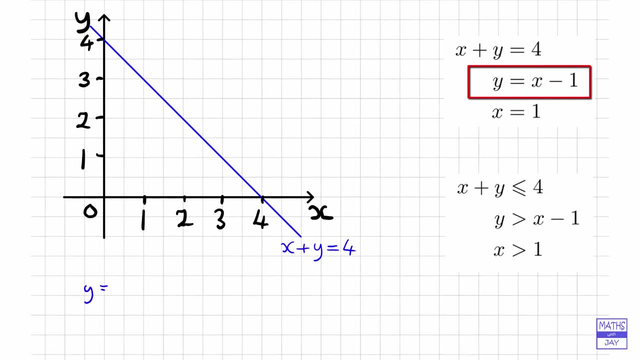 so there we've got. x plus y equals four. then let's think about the next line. so there we've got y equals x minus one. so one way of doing this one would be to choose a value for x and then work out what y is. so, for example, if x is two, then y is two minus one, so that's one. 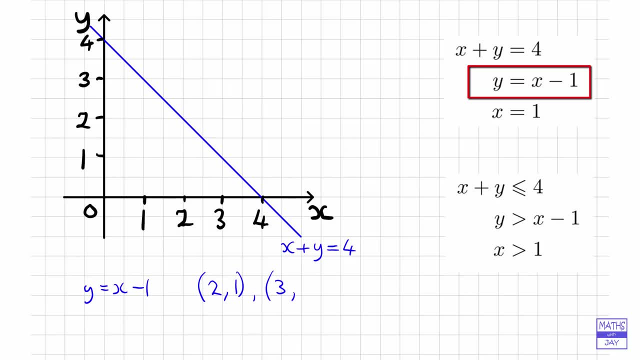 and if x is three, y will be three minus one, so that will be two and you only actually need two points for a straight line, but it's a good idea to do three just as a check. so if x is four, then y will be three. so those points are going to be two. one 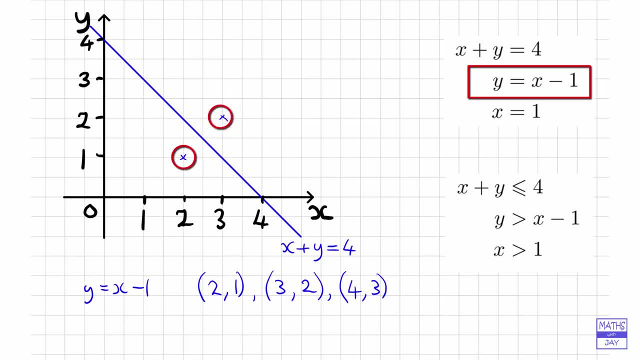 three, two and four, three, and then we just join those points and extend it in both directions. another way of thinking about drawing that line would be to say: well, we know that line is of the form: y equals mx plus c, and m is the gradient and m is the number multiplying the x. so that's one. 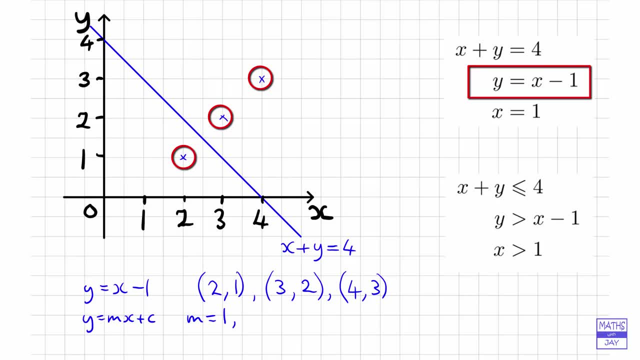 so we know that for every one along, we're going up one, and we know that c is equal to minus one, and that's where the graph cuts the y-axis. i'm just about seeing negative 1 on our graph, can't we? we can write it in there, so that's another way of drawing this graph. whichever, 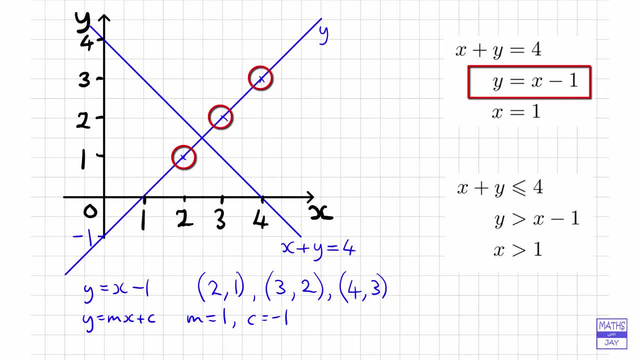 way you choose, it should come out to be the same thing. so that's the line: y equals x minus one. and then the last line is the simplest one, i think, because it's just x equals one. so we want the line. all the x values are equal to 1.. Once we've found 1 on the x-axis, we just draw a vertical line. 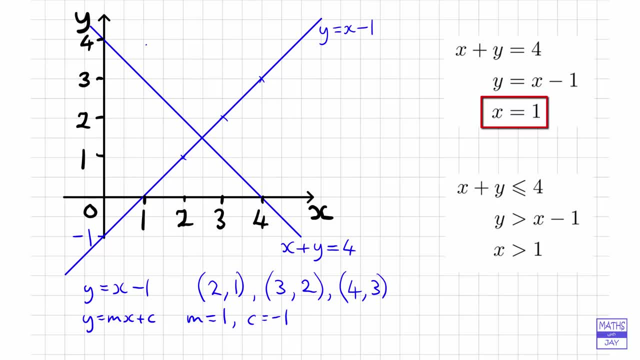 Any point on the line going through 1 vertically, so we could have that point there, for example, or point here. any point like that will be on that line. So that's the line x equals 1.. So that's part done. Now, in part, we're looking to show the region. 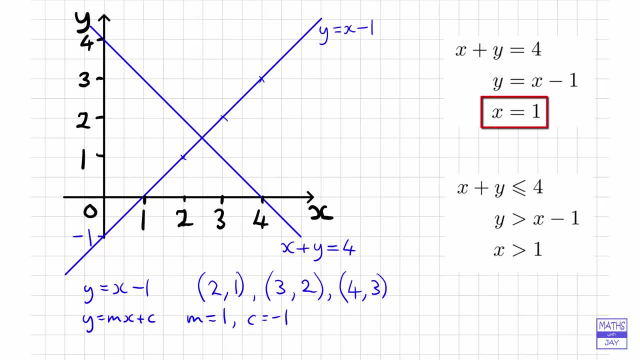 all the x values are equal to 1.. Once we've found 1 on the x-axis, we just draw a vertical line. Any point on the line going through 1 vertically, so we could have that point there, for example, or point here, any point like that will be on that line. So that's the line. x equals 1.. 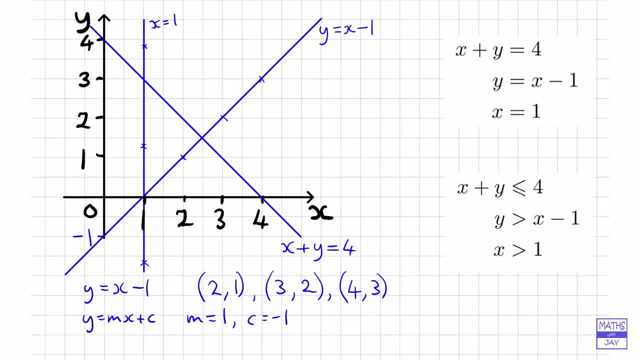 So that's Part A done. Now in Part B we're looking to show the region that's satisfied by these 3 inequalities Now, because we've got, or in one of the lines, that's easy, because that's going to require a solid line. but the other two both have greater than. 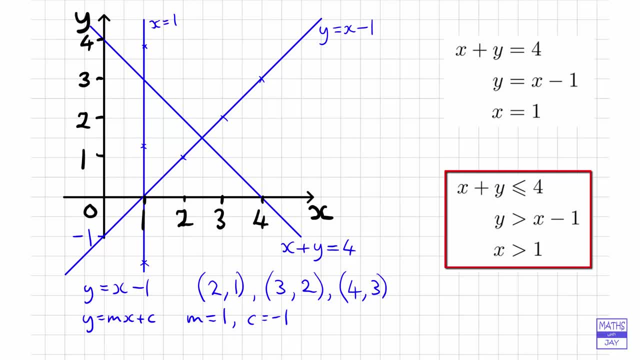 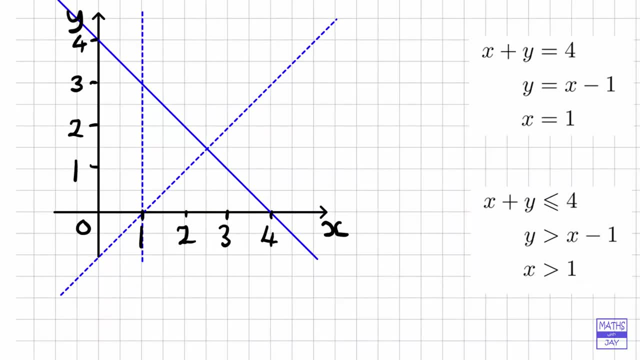 as they don't have equal, so we don't want to include the line, so we need those to include dotted lines. so let's have a look at what that will look like. So, because in x plus y is less than or equal to 4, we've got the equals. that's a. 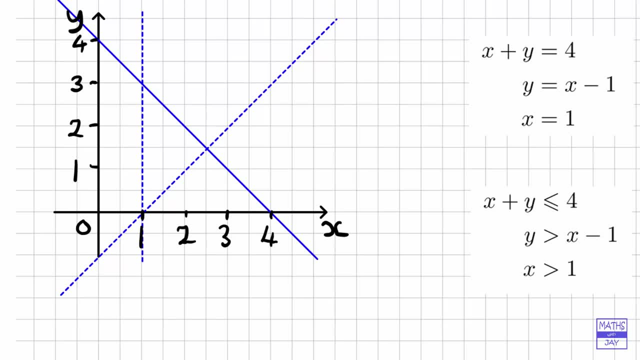 solid line, but the other two have not got equals. so for y equals x minus 1, we've got the line looking like a dotted line, and the same for x equals 1, because we don't want the lines included. So now what we need to do is shade the 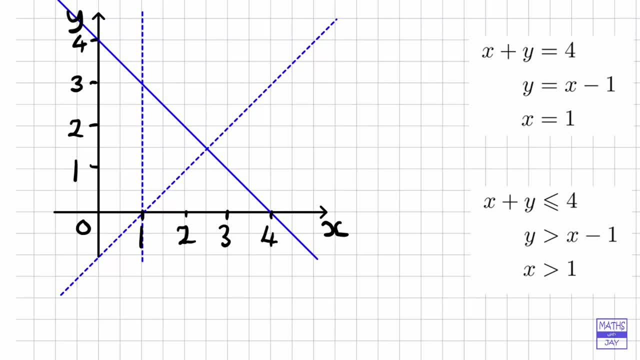 region that we don't want, so that we end up with the region that we do want and then we can write the letter R in there, Right? so we want to first of all look at: x plus y is less than 4. so the region we don't want is x plus y is greater than. 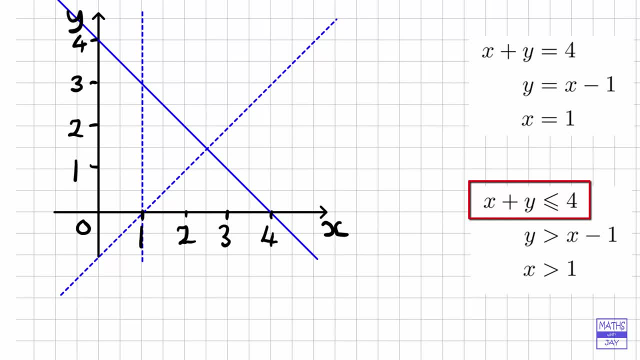 4. so we want to shade out the area above that line. so we're getting rid of all of that. So we can choose any point in that region and check that x plus y does add up to something greater than 4 in the area that we've shaded out. so for 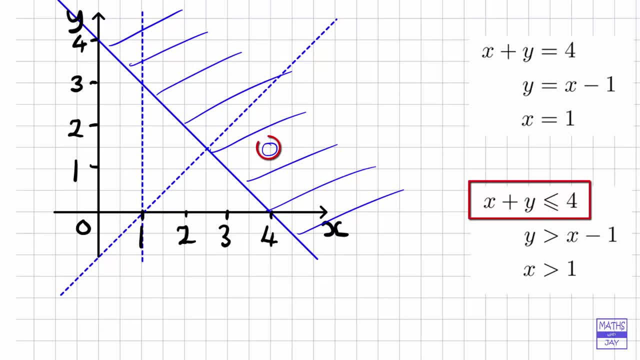 example, if I choose this point here, x is 4 and y is 1.5. if we add those together we get 5.5. so that's greater than 4. so that's good. we don't want that point, Right? so then let's have a look at some. y is greater than x minus 1, so now we 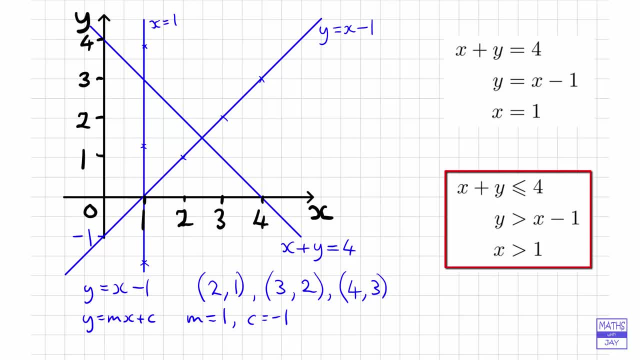 that's satisfied by these three inequalities. Now, because we've got less-than or equal-to in one of the lines, that's easy because that's going to require a solid line. but the other two both have greater than, so they don't have equals, so we don't want to include the line. 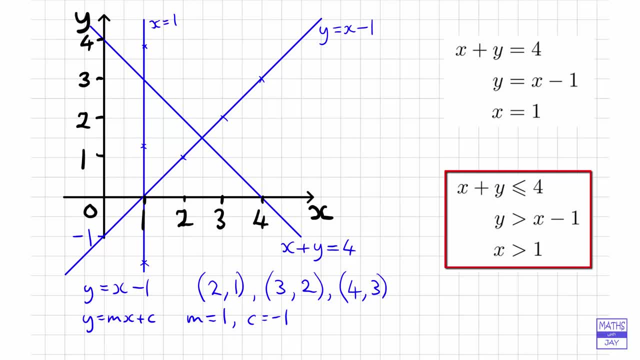 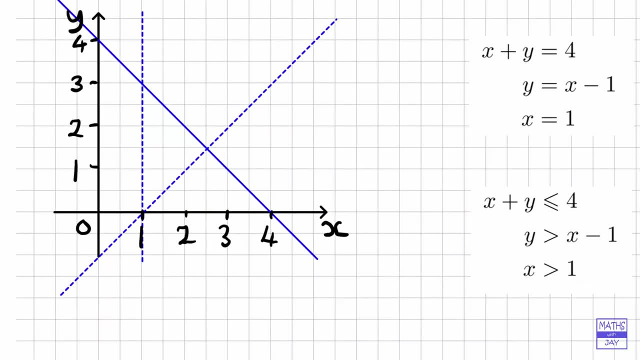 so we need for that to be less than or equal to 1.. those to include dotted lines. so let's have a look at what that will look like. So, because in x plus y is less than or equal to 4, we've got the equals. that's a. 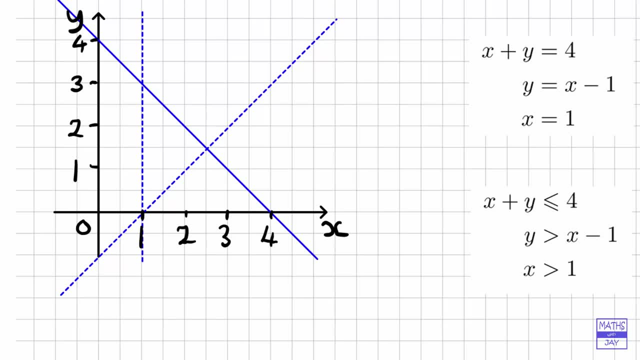 solid line, but the other two have not got equals. so for y equals x minus 1, we've got the line looking like a dotted line, and the same for x equals 1, because we don't want the lines included. So now what we need to do is shade the 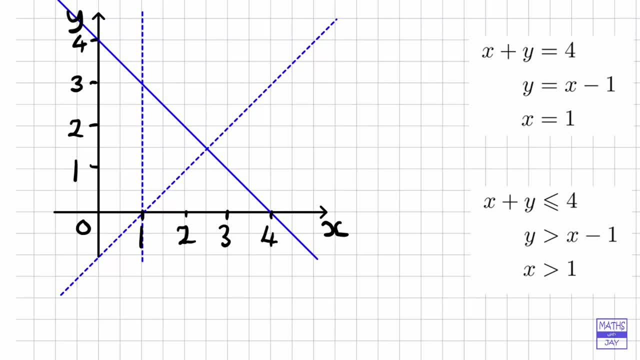 region that we don't want, so that we end up with the region that we do want and then we can write the letter R in there, Right? so we want to first of all look at: x plus y is less than 4. so the region we don't want is x plus y is greater than. 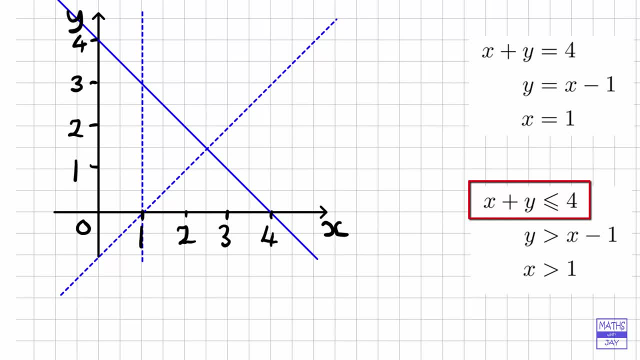 4. so we want to shade out the area above that line. so we're getting rid of all of that. So we can choose any point in that region and check that x plus y does add up to something greater than 4 in the area that we've shaded out. so for 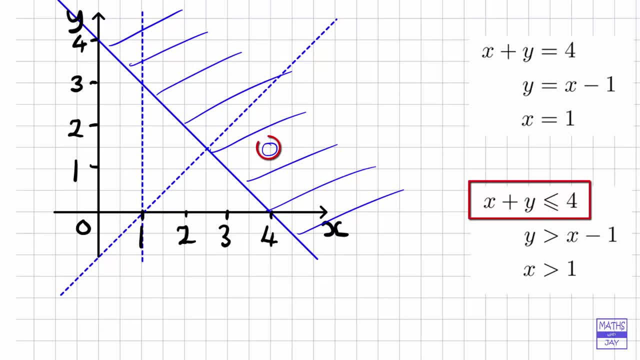 example, if I choose this point here, x is 4 and y is 1.5. if we add those together we get 5.5. so that's greater than 4. so that's good. we don't want that point, Right? so then let's have a look at some. y is greater than x minus 1, so now we 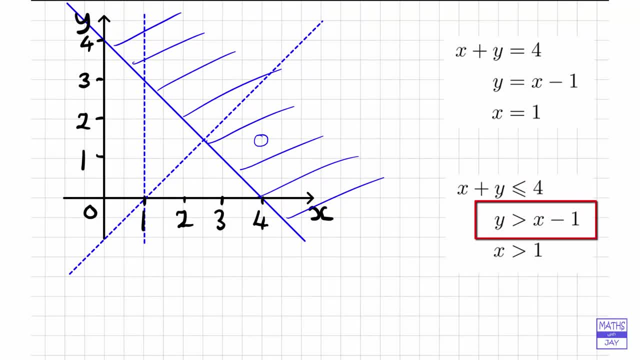 want to shade the area where y is less than x minus 1. so we want to shade the area underneath that line. so that's down here. so we're shading out all of that. that's the bit we don't want again. we can check that we've shaded out the. 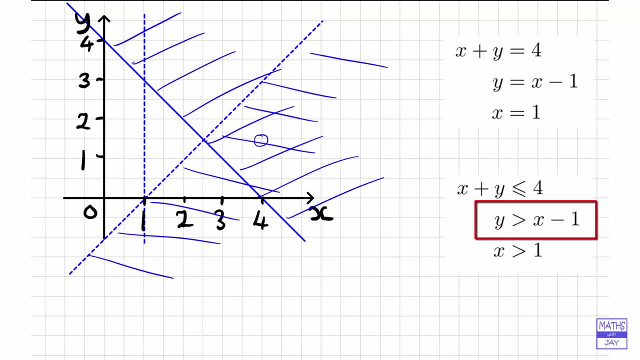 right area. so let's have a look at what should we take. let's take a point on the axis. so the point when x is 3 and y is 0, so if y is 0 and x is 3 and 3 minus 1, is: 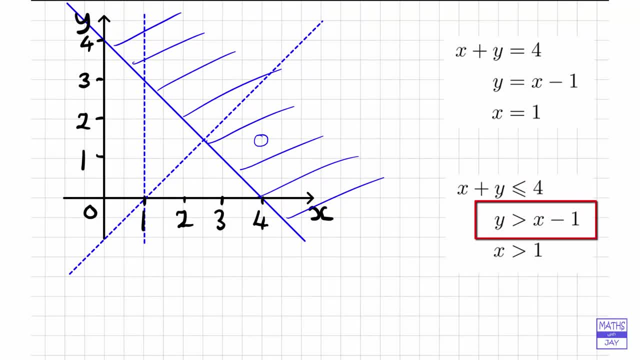 want to shade the area where y is less than x minus 1. so we want to shade the area underneath that line. so that's down here. so we're shading out all of that. that's the bit we don't want again. we can check that we've shaded out the. 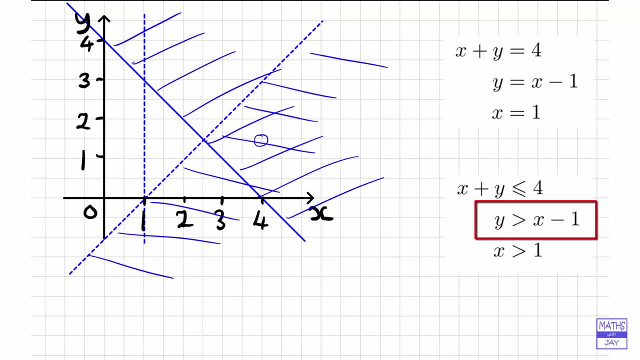 right area. so let's have a look at what should we take. let's take a point on the axis. so the point when x is 3 and y is 0, so if y is 0 and x is 3 and 3 minus 1, is: 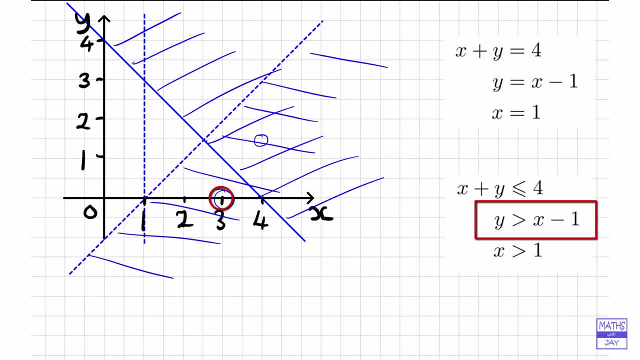 2, so 0 is not greater than 3 minus 1, so 0 is not greater than 2. so that's good. we don't want that point. and finally, we're going to look at the line: x equals 1 and we want to shade out where x is. 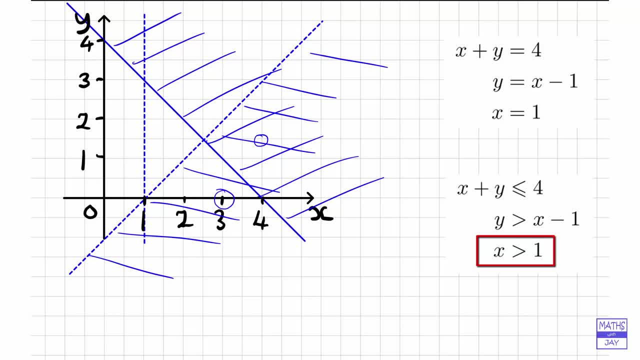 less than 1, because we want where x is greater than 1. so let's do the left-hand side of that line that we're shading Again, we can check. take a value, any value to the left of that line, and x will be less than 1. so that's the right. 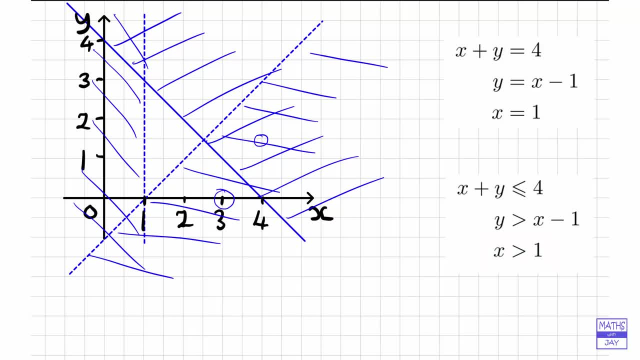 area. so you can see that we're left with one area. we're going to label with the letter R, which we do want, So you should find, if you choose any point inside there, that it does satisfy all three of those inequalities. So let's just choose one point. So, as I'll check, we're looking at. 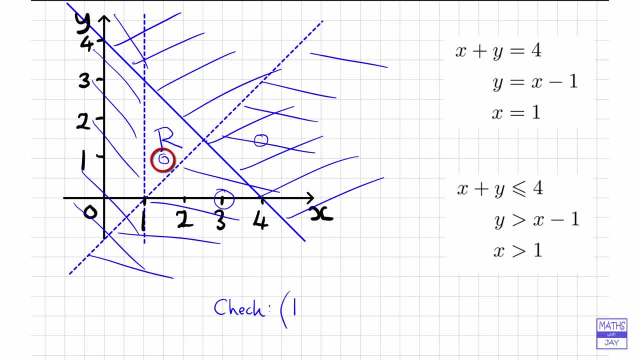 the point with coordinates. where do I circle there? the point x is one and a half and y is one. So we should find all three inequalities are satisfied for that point. So one and a half plus one. looking at our x plus y, that's two and a. 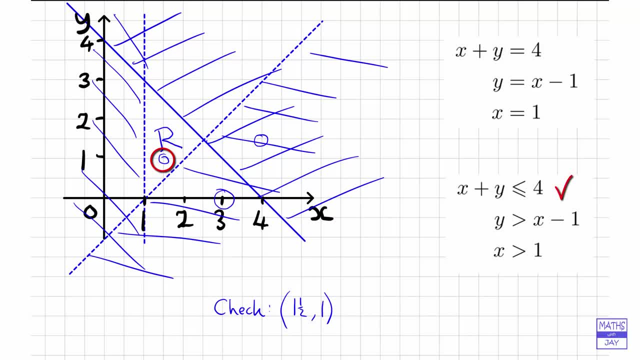 half, so that is less than four. that's fine. If we subtract one from x, we get a half, and then one is greater than half. so y is greater than x minus one and x is greater than one because it's one and a half. so that looks fine. Thank you.